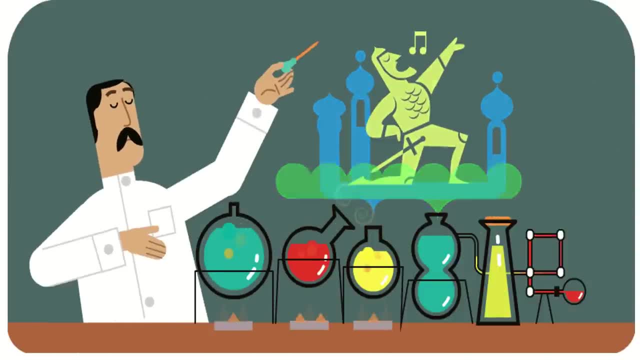 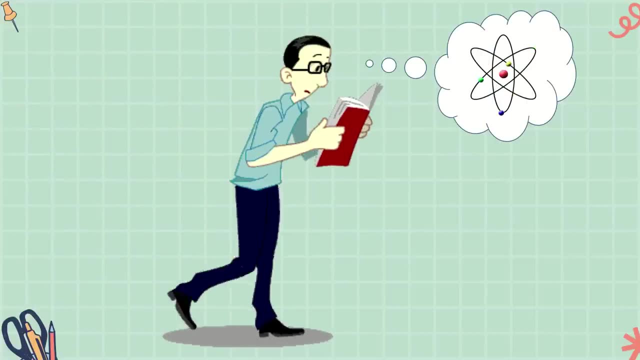 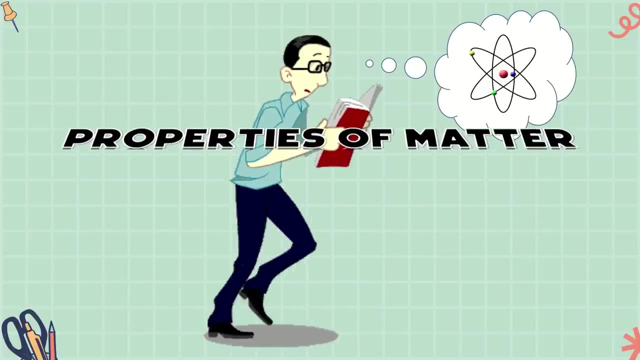 When you were in Grade 7, you learned to classify substances into elements, compounds and mixtures. Now you will be on a magical journey Because we will be studying the properties of matter. Are you excited? class, Let's go. 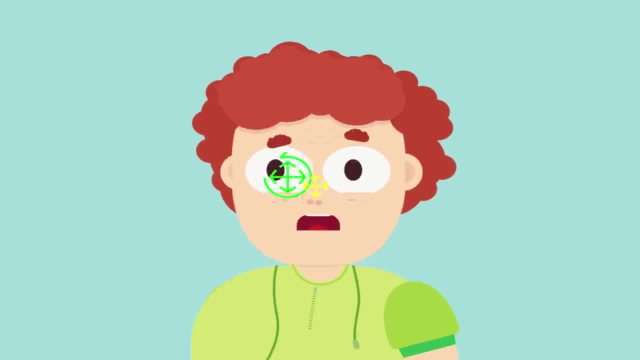 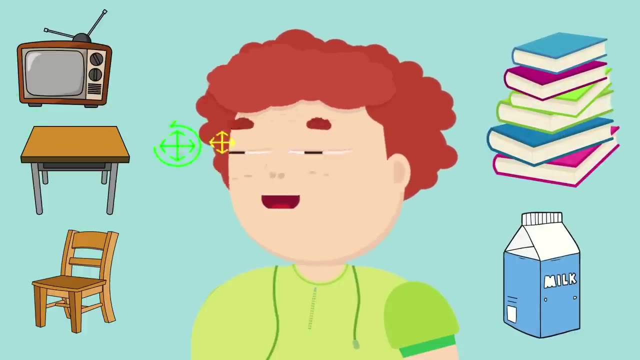 Look around inside your house, You can see a variety of things such as television, table, chair, book, carton of milk and many more. What do you think are the similarities of the things mentioned? You're right, They are all examples of matter. 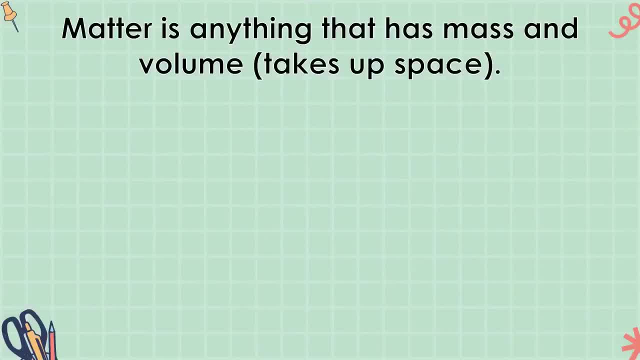 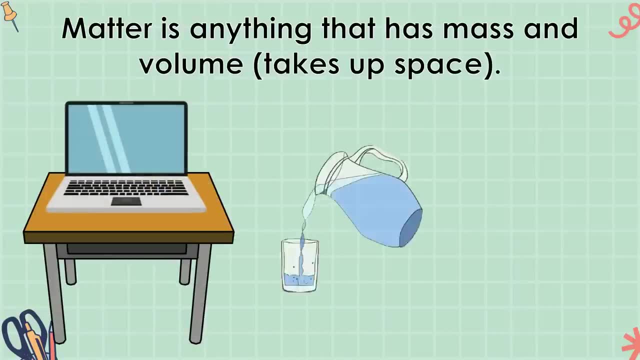 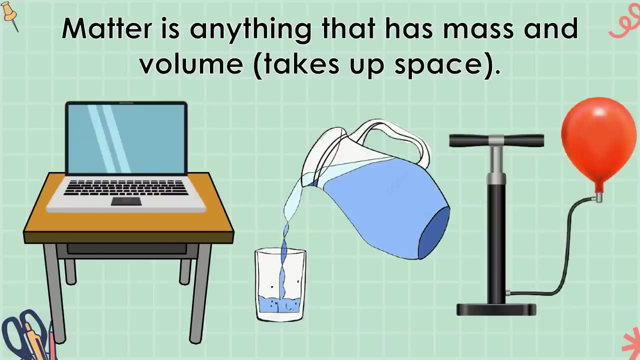 Matter is anything that has mass And volume And it takes up space. For example, if you put your laptop on the table, or you put water in a glass or you blow on a balloon, all of them occupy space. In other words, all of them are examples of matter. 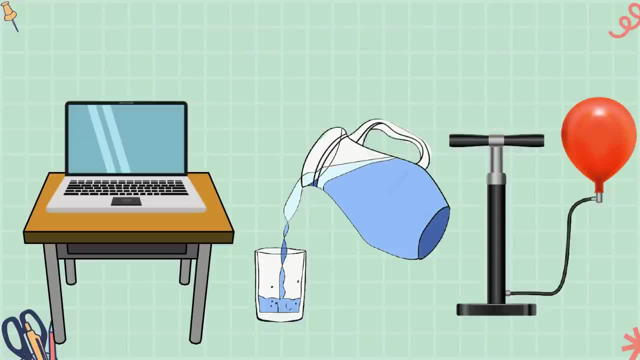 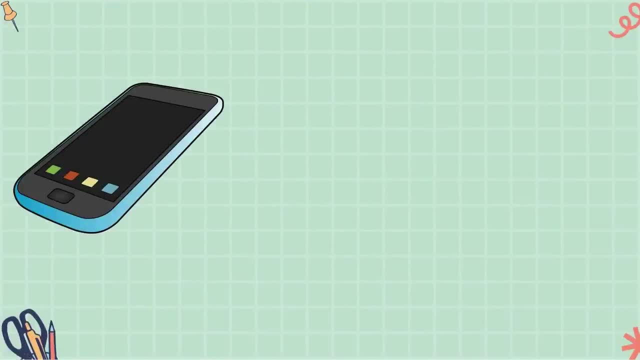 Remember class that matter occupies space. Volume is a measure of the space occupied by an object. Now try to understand the properties of matter. What are the strengths and weaknesses of a cell phone? It depends on the machine. And last, the can of soda. 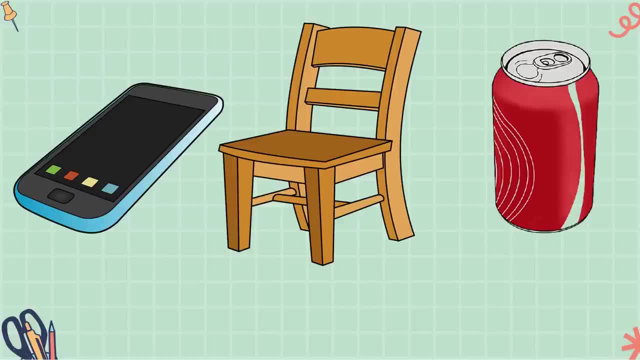 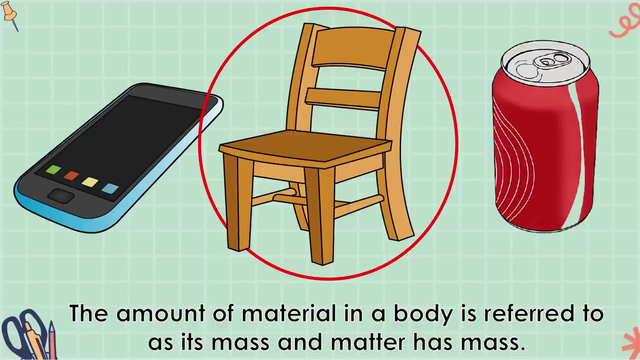 Which one is heavier? If your answer is chair, then you are correct. It is heavier compared to the cell phone and the can of soda. But why? Because its mass is greater. We should always remember that the amount of material in the body is referred to as its mass. 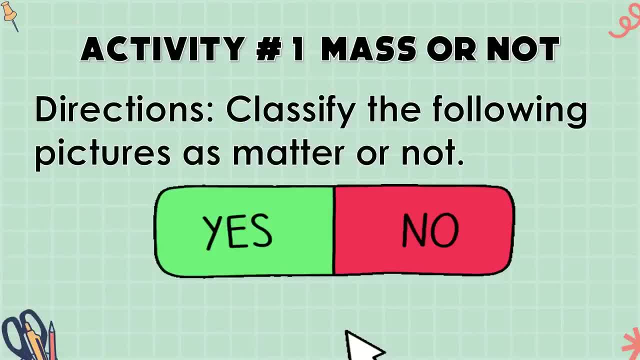 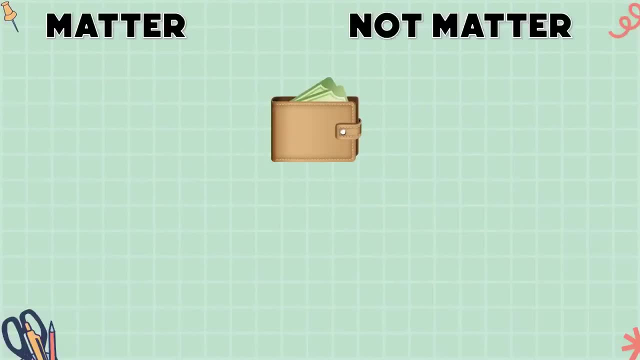 And mater has mas. Now let us try this activity. Mas or not, Classify the following pictures as mater or not. Are you ready? Let's answer. Let's have the first picture, Wallet. is it a mater or not? 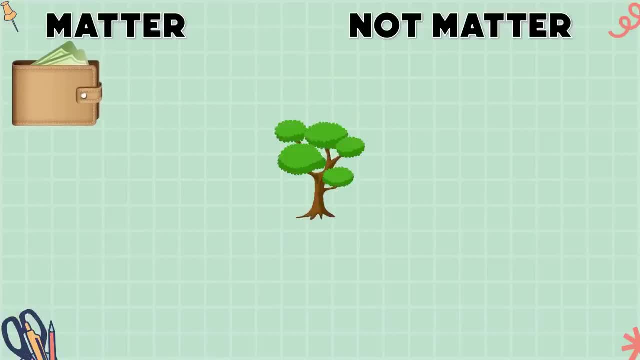 Mater. that's right Next tree O puno. ito ba ay mater o hindi? Tama ka? ito ay kabilang sa mater. Sumunod Heat. ito ba ay mater o hindi? Tama ka uli? ito ay hindi mater. 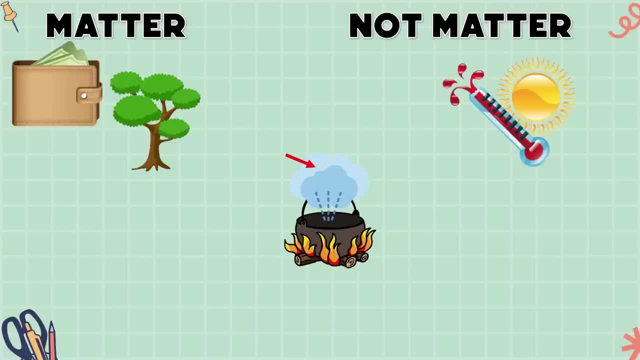 Next water vapor or steam? Ito ay mater. Sumunod naman hangin sa loob ng inflatable pool. Ito ay kinukonsiderang mater. That's right, Viligar o suka, ito ba ay mater o hindi? 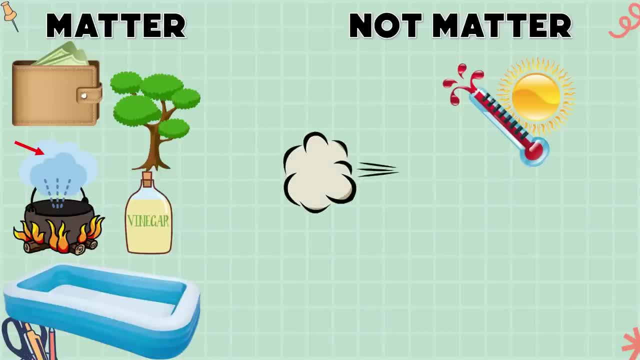 Ito ay mater din Next smoke o usok. Ito ay mater Tama Panghuli light. Ito ba ay mater o hindi. This is not a mater That is correct. Based on this activity, we can say that all our answers in the mater column can be measured. 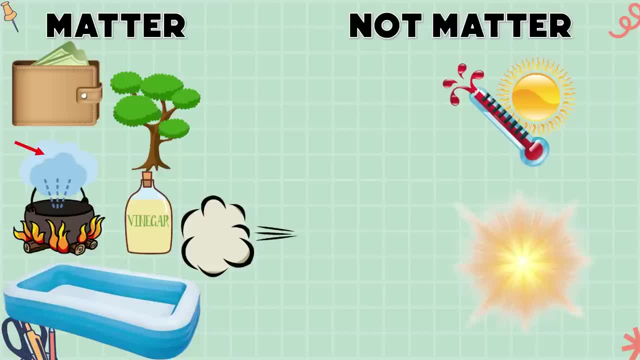 Lahat sila ay maaaring masukat. Bakit? Because mater occupies space and has mass. Paano naman ang heat at light? Do they occupy space? The answer is no, They do not occupy space and don't have mass. 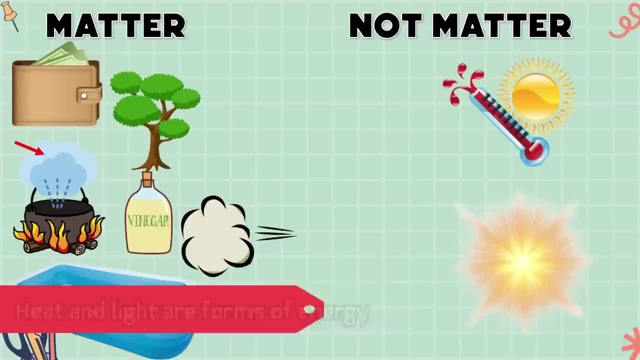 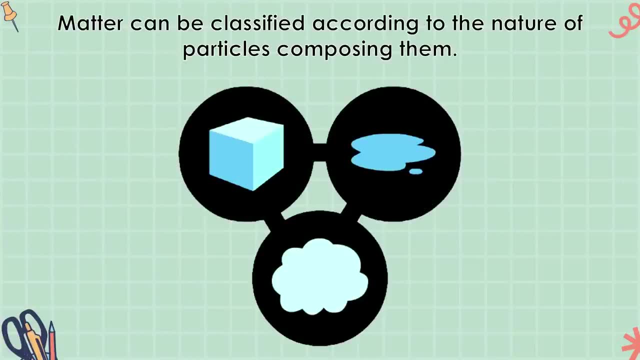 Sa makatawid hindi sila matatawag na mater. Heat and light are forms of energy And in chemistry, energy is not a mater. Mater can be classified according to the nature of particles composing them. In class, they are classified as solid, liquid and gas. 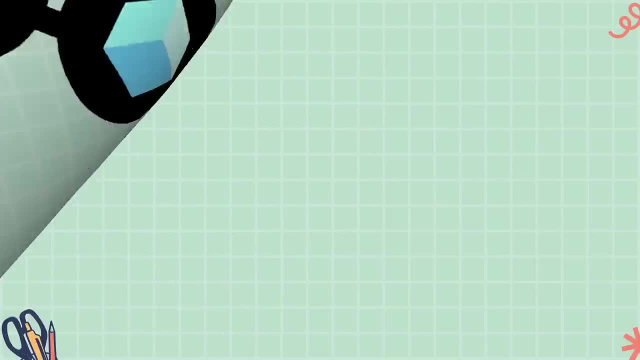 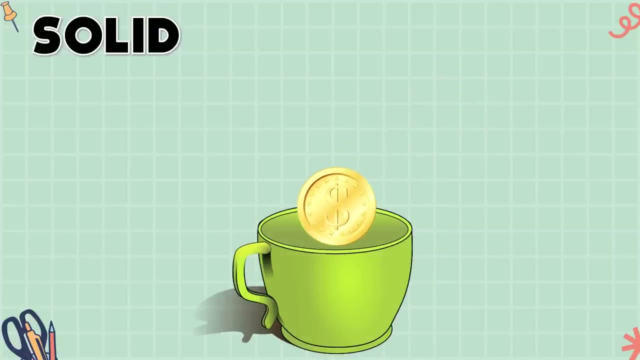 Tara at isa-isahin natin silang pag-aralan Solid. Try putting a coin into a cup. May nangyari ba sa shape or size ng coin? Wala, The coin keeps its original shape. The coin keeps its original shape. 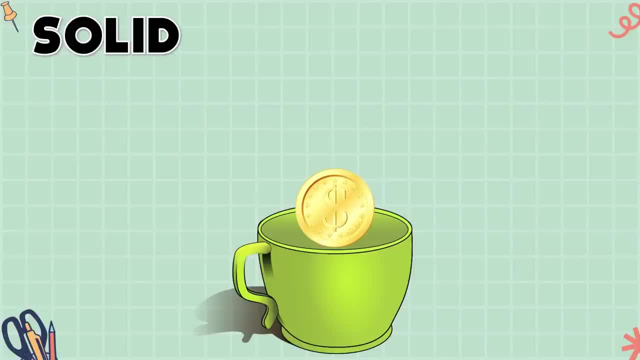 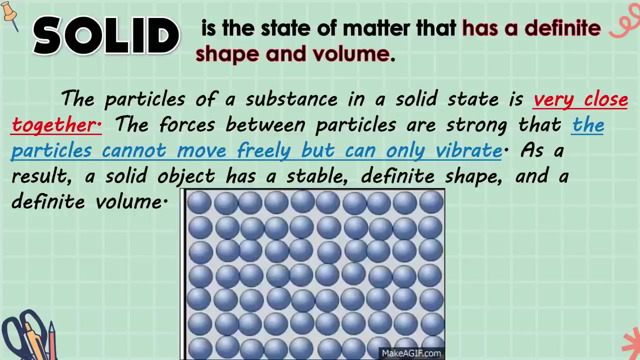 The coin keeps its original shape and volume. Pero bakit? Because the coin is solid. We can define solid as the state of matter that has a definite shape and volume. The particles of a substance in a solid state is very close together. The forces between particles are strong that the particles cannot move freely but can only vibrate. 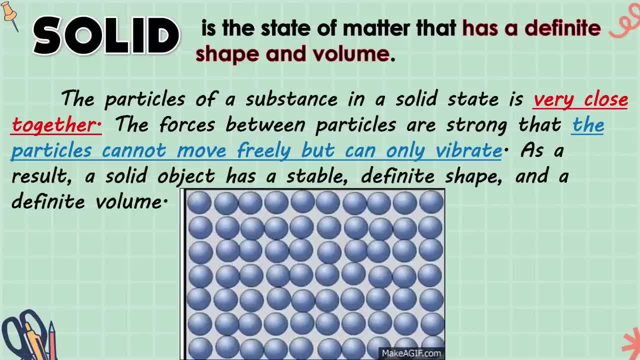 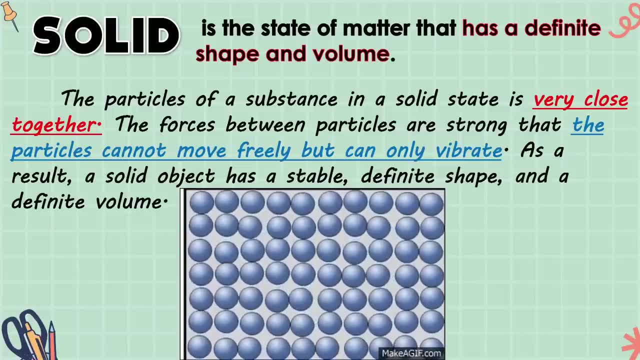 Look at the picture class. As a result, a solid object has a solid shape. A solid object has a stable, definite shape and a definite volume. Ang ibig sabihin ito: ang solid ay kayang i-maintain ang kanyang shape at volume kahit na ilipat pa ito sa ibang container. 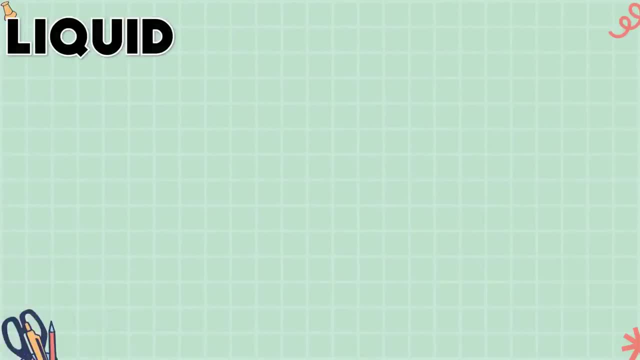 Next is liquid. Subukan naman nating magsalin ng orange juice from a pitcher to a glass. Did the orange juice take the shape of the glass? Yes, Yes, Nagiba ba ang volume ng orange juice. Paano naman ang lasa nito. 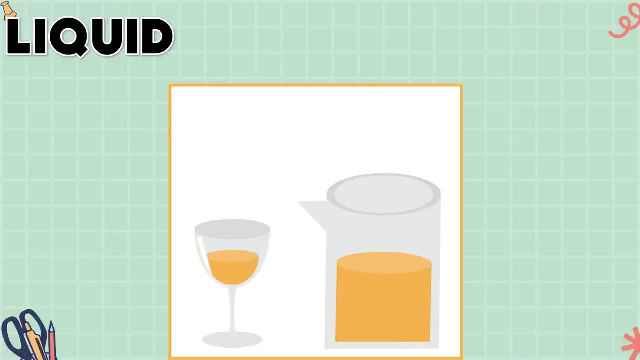 Nagbago rin ba Hindi Magaling Nang isali ng orange juice sa baso. ang tanging bagay na nabago ay ang kanyang shape. Nagbago ito dahil ang orange juice ay isang liquid. 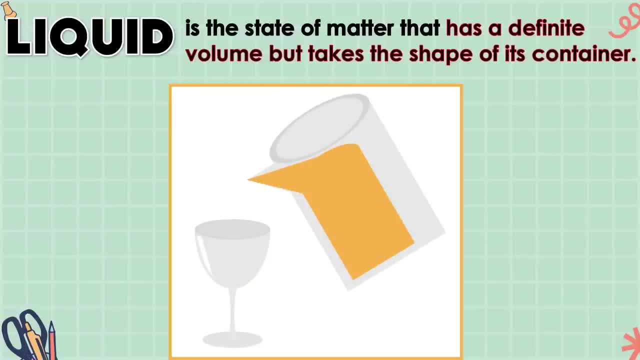 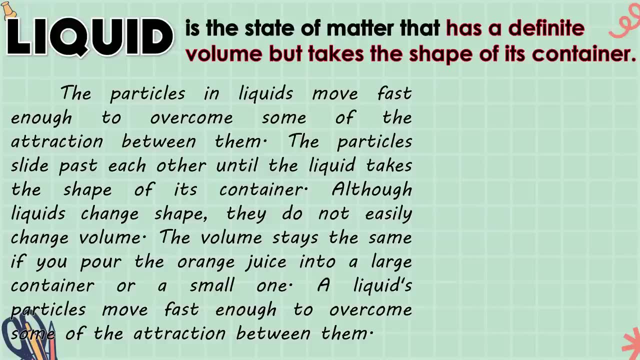 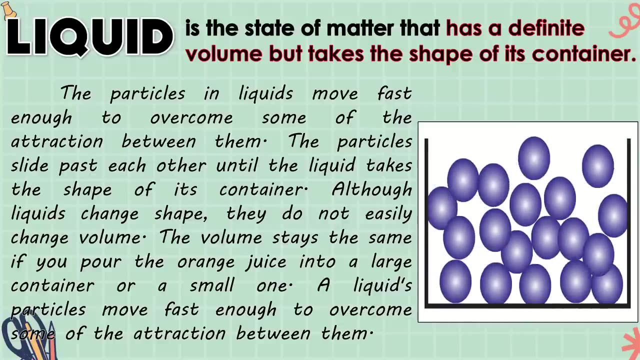 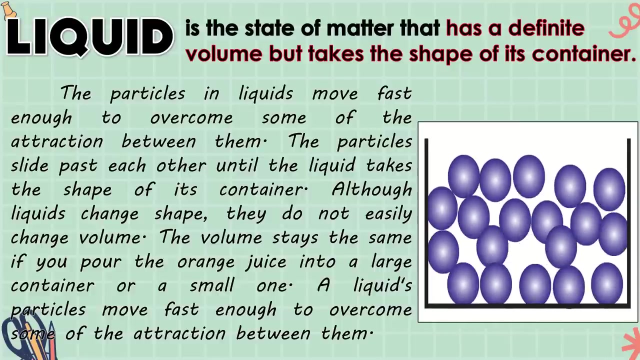 Liquid is the state of matter that has a definite volume but takes the shape of its container. The particles in liquids move fast enough to overcome solid state. The particles slide past each other until the liquid takes the shape of its container. Although liquids change shape, they do not easily change volume. 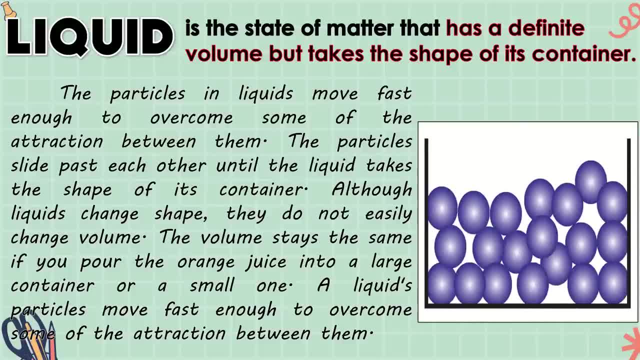 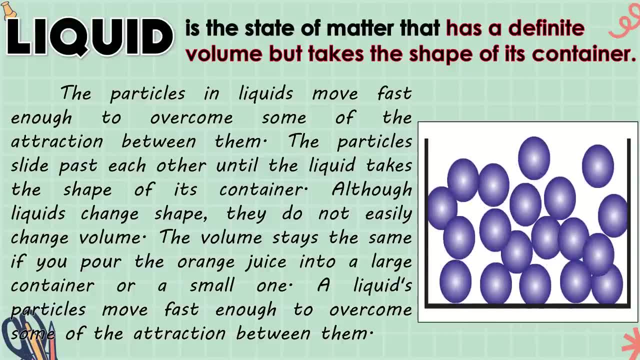 Ang volume ay mananatili, kahit na isalin pa ito sa mas malaki o mas maliit na lalagyan. As you can see in the picture, a liquid's particles move fast enough to overcome some of the attraction between them. 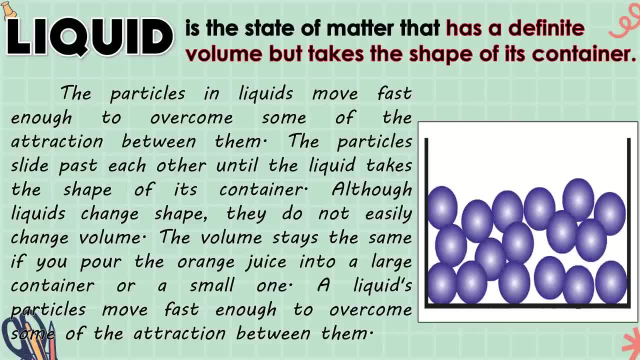 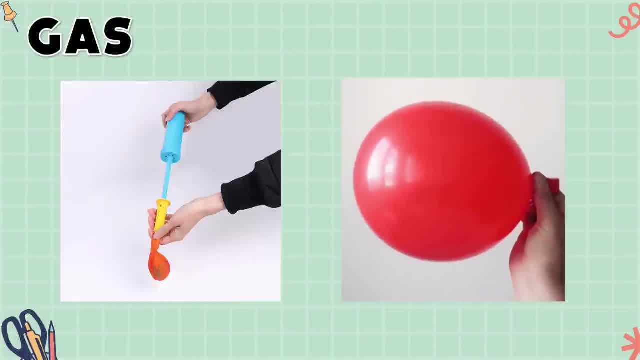 That is liquid At ang panghuli ay ang gas. Nasubukan mo na bang mag-inflate o mag-deflate ng lobo. What have you observed? We can say na ang baloon ay mag-i-inflate kapag nilagyan ito ng hangin sa loob, at ito naman ay magde-deflate kapag ito ay pinres o binitawan, at ang hangin sa loob ng lobo ay lalabas. 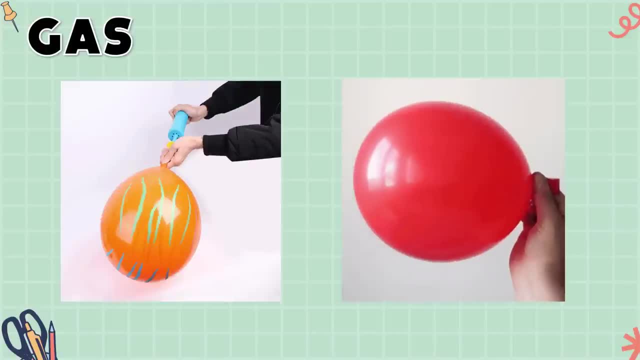 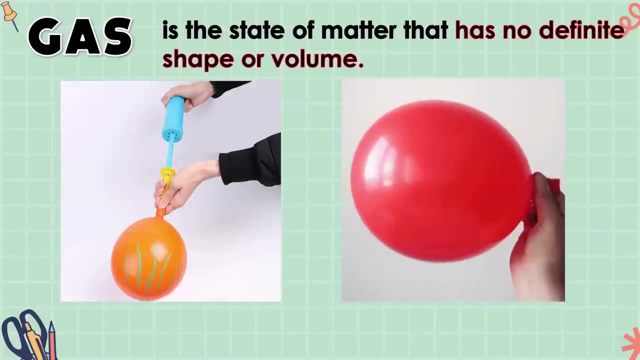 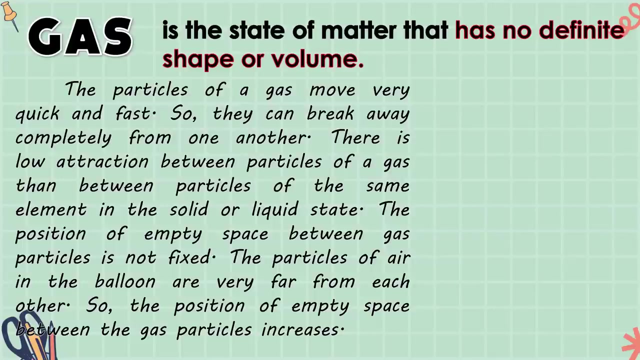 Ngunit bakit naman? Ngunit bakit kaya? It is because of the state of matter called gas, And gas is the state of matter that has no definite shape or volume. The particles of a gas move very quick and fast, so they can break away completely from one another. 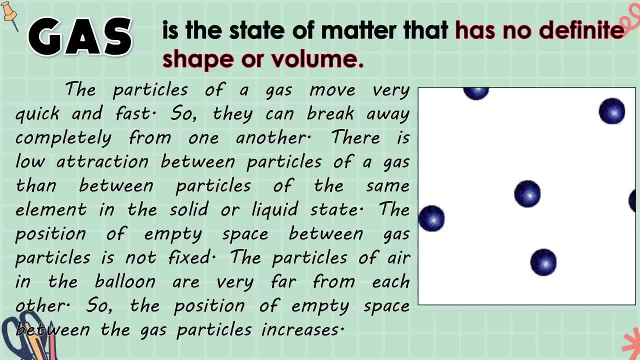 Check out this picture. class Mababa ang attraction between particles ng gas than between the particles of the same element in the solid or liquid state. The position of the empty space between gas particles ay hindi fixed. Kaya naman ang mga particles ng air sa loob ng baloon ay magkakalayo sa isa't-isa.